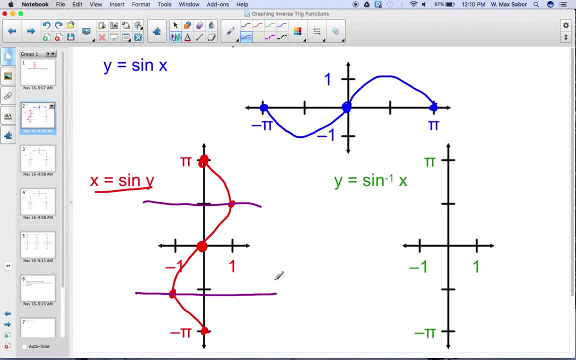 fail the vertical line test. So what we typically will do is restrict it between pi over 2 and negative pi over 2.. So this will create our arcsine function that goes from 1 comma pi over 2 down to the origin And then that goes. 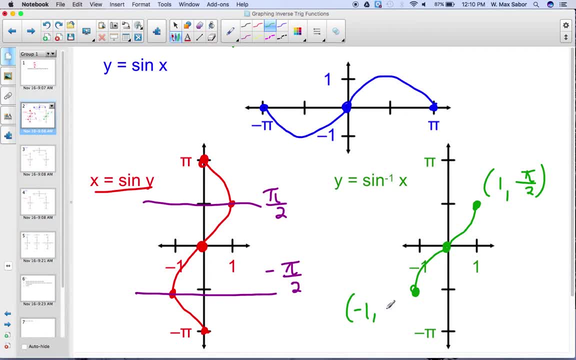 to negative 1 comma, negative pi over 2.. You do need to know what these points are And you also need to know that this is not straight. This should be curving up and then curving down. Let's do cosine now. Cosine starts at a maximum, goes to equilibrium and then a minimum. 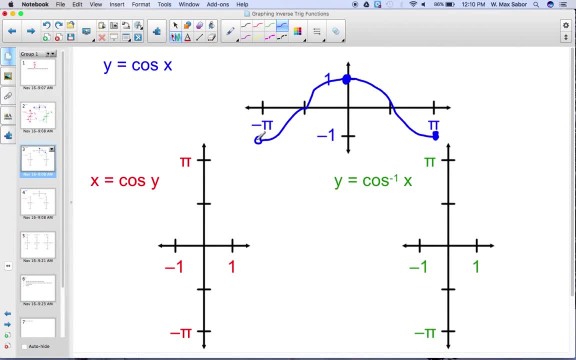 In the other direction it goes to equilibrium, then minimum. So if we reflect that over a diagonal we'll be switching x and y. So 0 comma 1 becomes 1 comma 0. Here are our points. So hopefully you agree that this is what x equals cosine of y would look like. 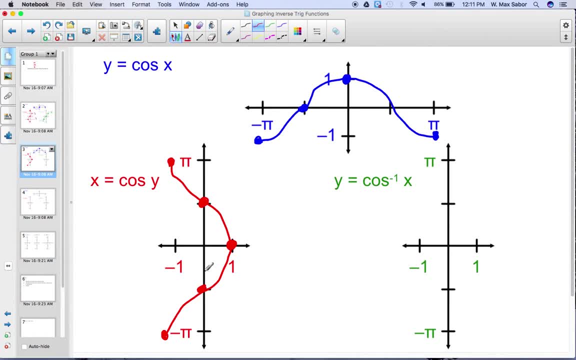 But this is not. This is still not a function Because it doesn't pass the vertical line test. If we did the same restriction between negative pi over 2 and pi over 2, we still would fail the vertical line test. So we need to go from 0 to pi here. 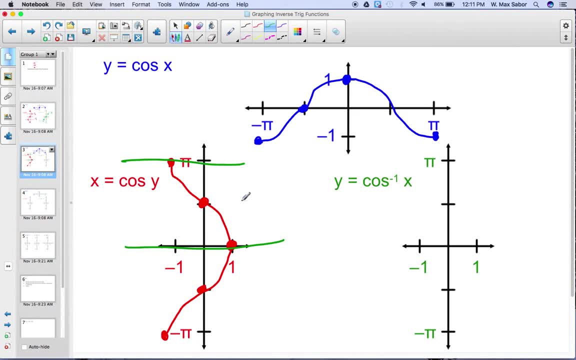 So we'll go from pi down to 0.. So, starting there, Going backwards To negative, 1 comma pi, And this is 1 comma 0. This is 0 comma pi over 2.. What does tangent look like? Tangent starts at equilibrium and has asymptotes.